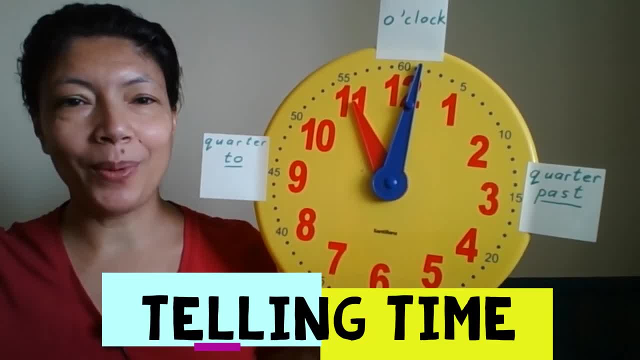 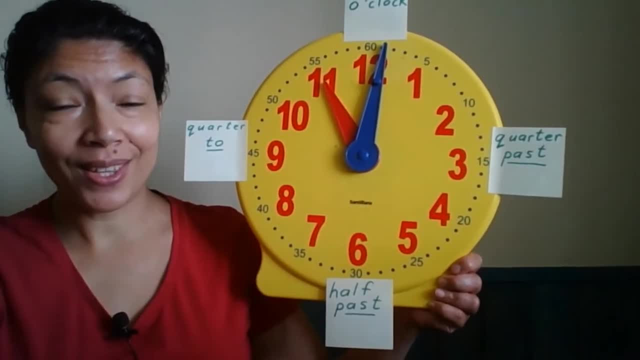 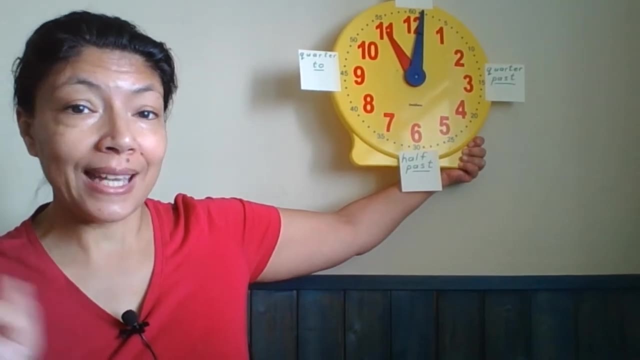 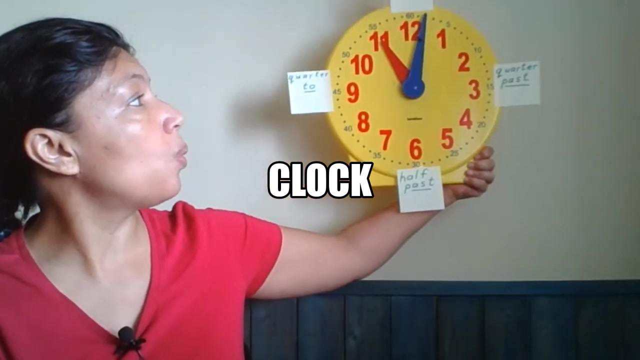 Hello, Today we are going to learn to tell time. This is a clock. This is a clock, We put it on the wall. It isn't a watch that we put on our wrist. We put a clock on the wall. Alright, on the clock. 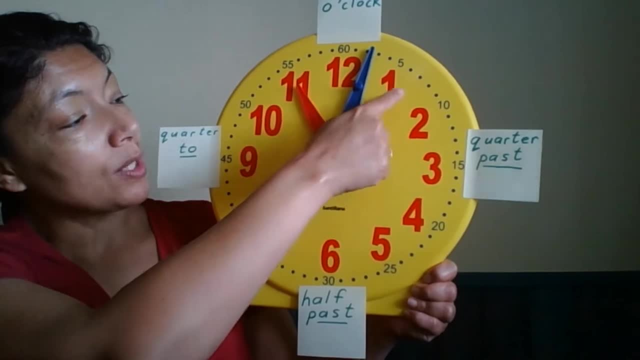 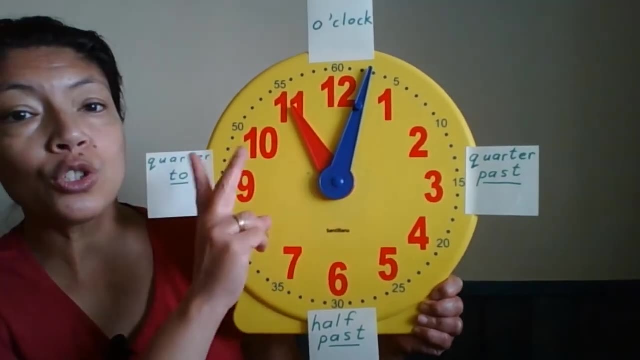 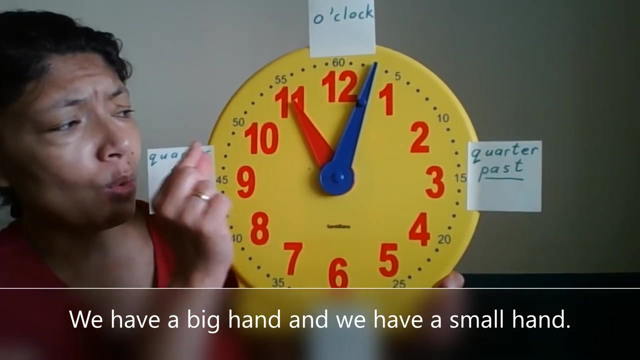 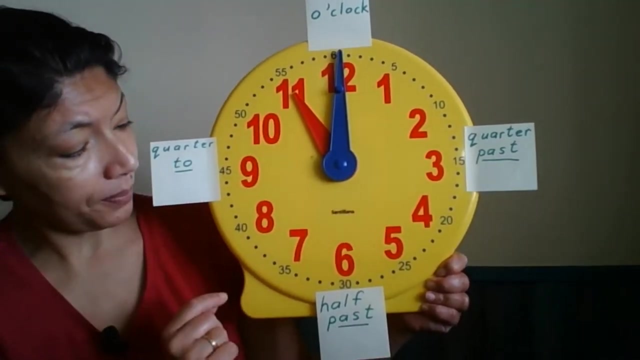 we have numbers 1,, 2,, 3,, 4,, 5,, 6,, 7,, 8,, 9,, 10,, 11 and 12, and we have two hands. We have the big hand, this blue one, and we have a small hand, this red one. Let's see how this works, Where the 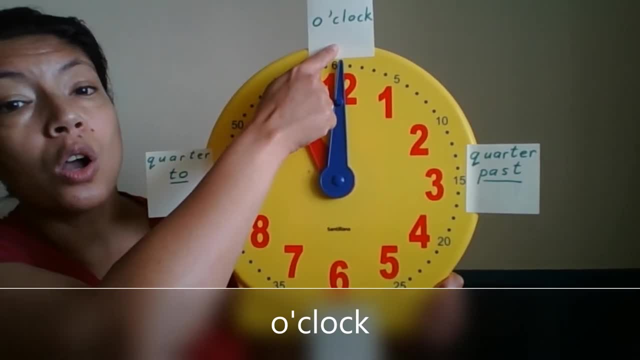 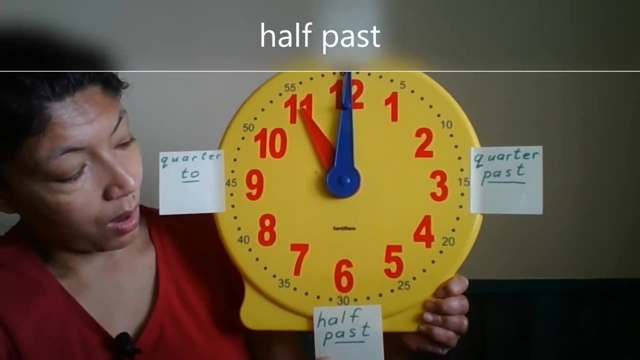 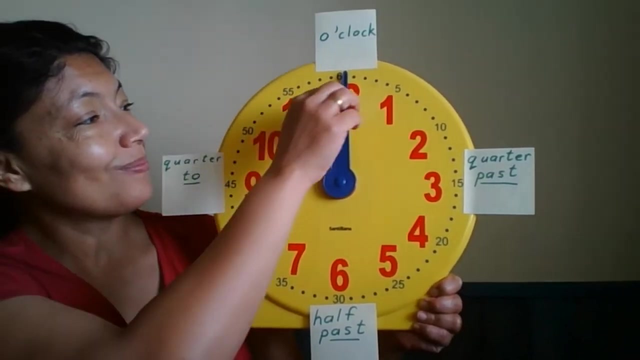 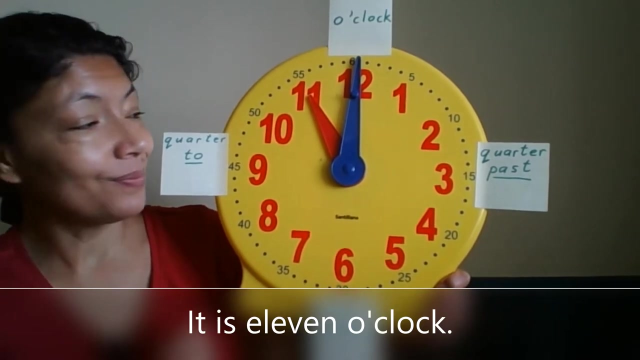 12 is. it is o'clock. Quarter past, half past, quarter to Now. it is 11 o'clock. 11 o'clock. The small hand is on the wall. Let's see how this works. We put a clock on the wall. It isn't a. 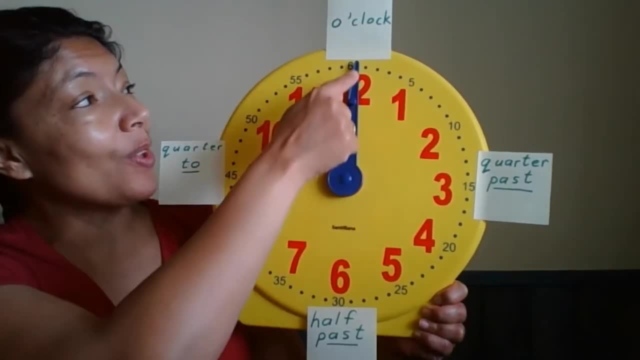 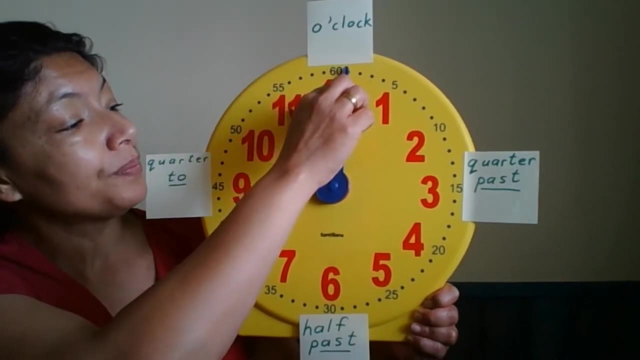 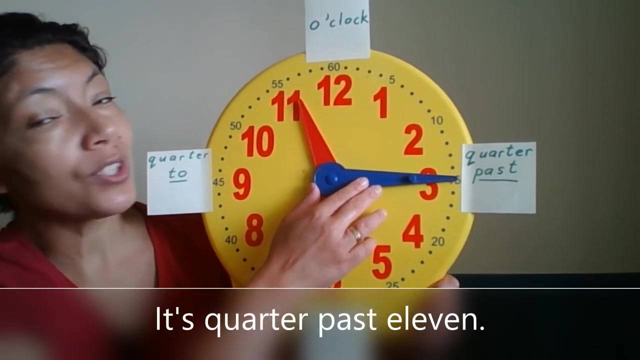 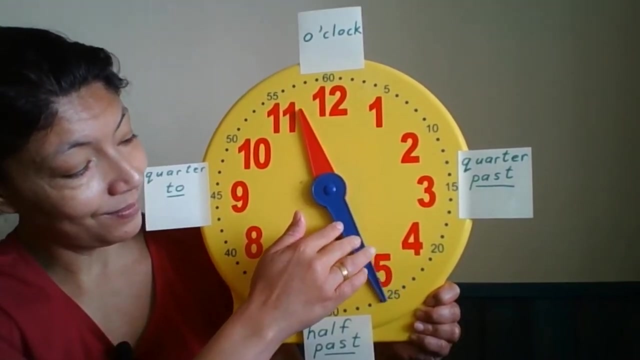 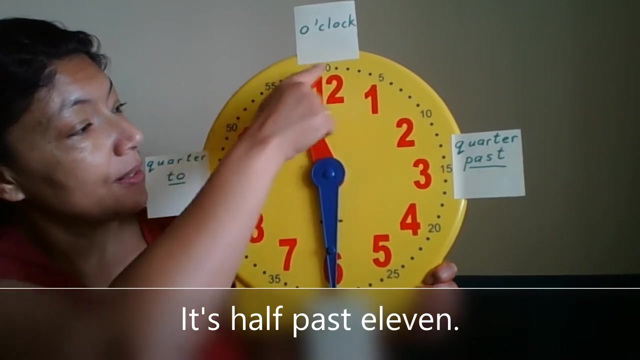 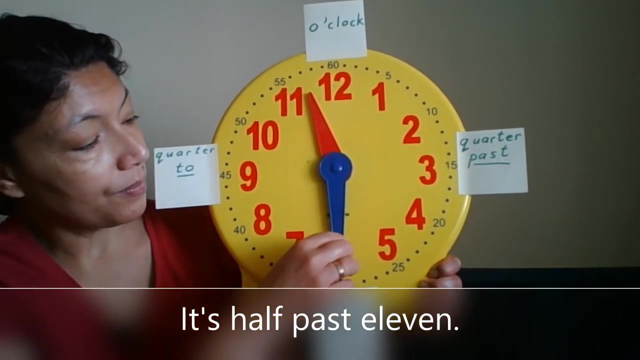 the 11.. The big hand is on the 12.. So it is 11 o'clock, It's quarter past 11.. It's quarter past 11.. It's half past 11.. It's half past 11. Past. 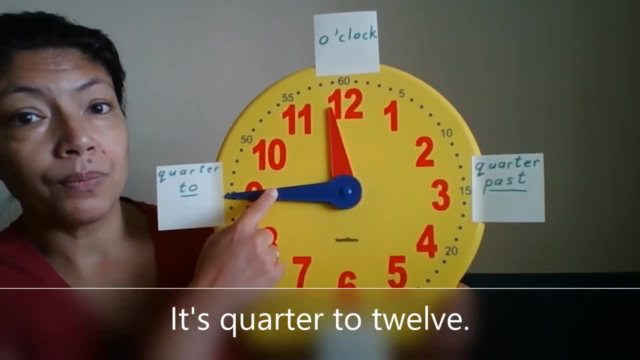 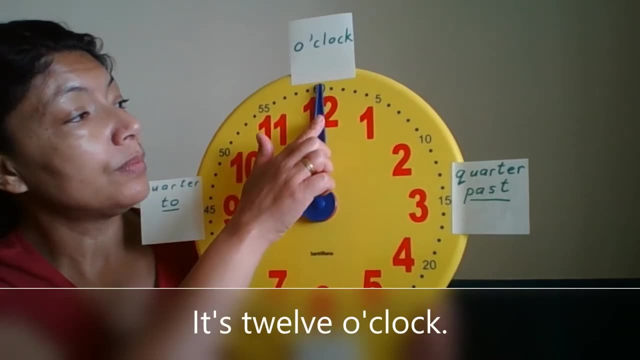 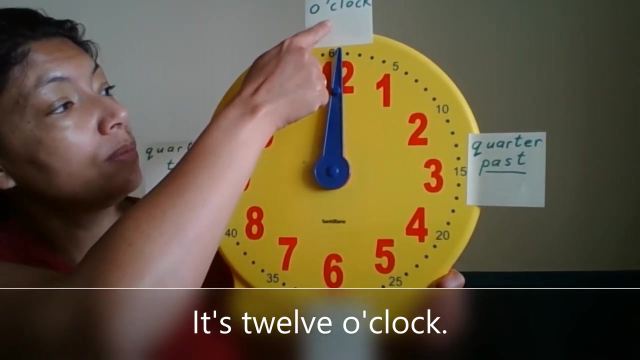 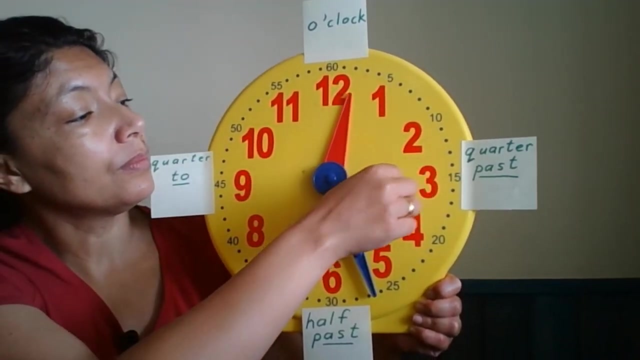 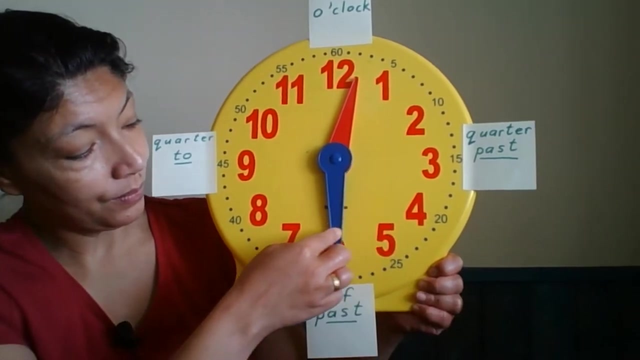 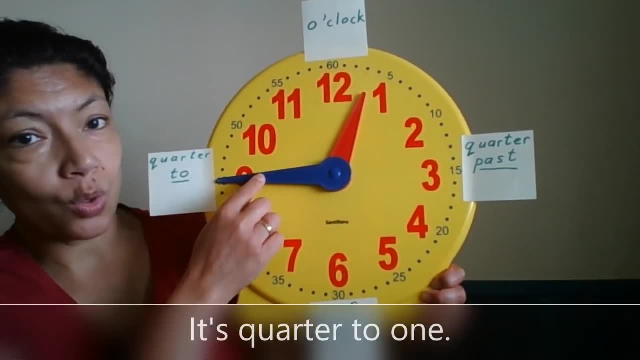 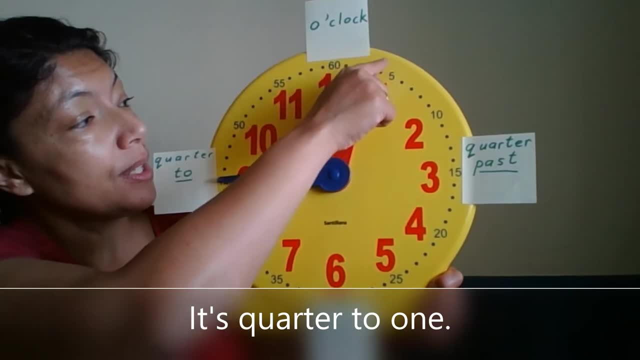 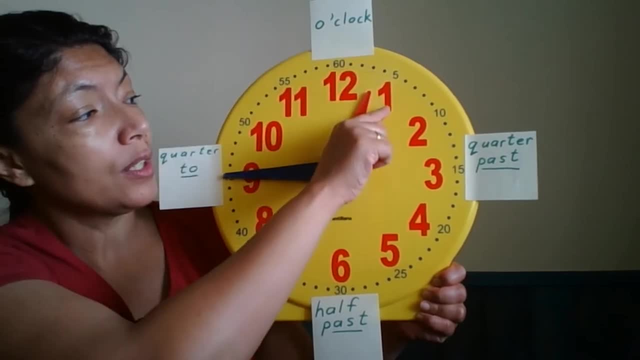 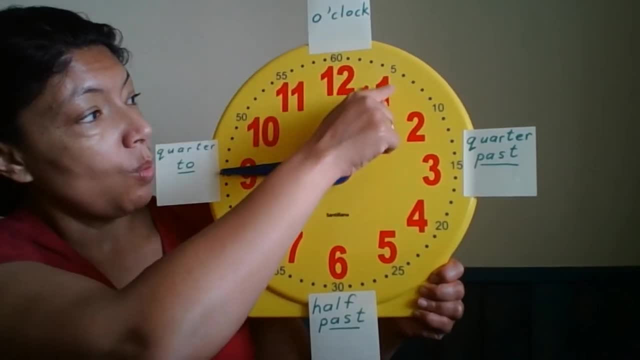 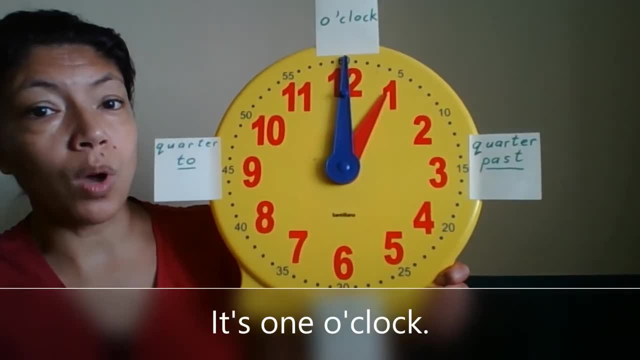 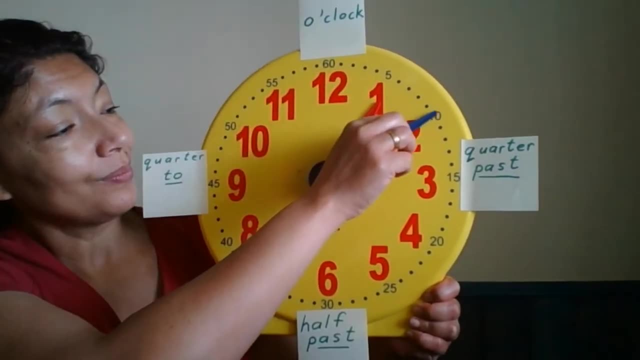 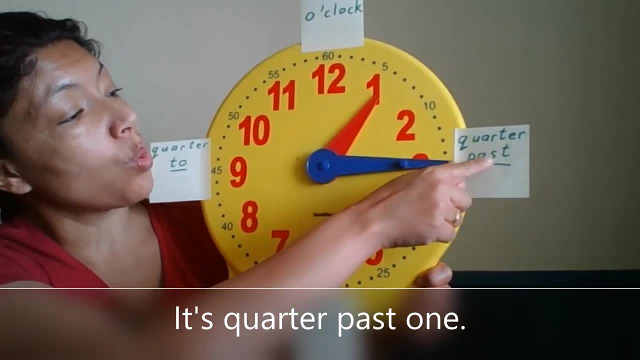 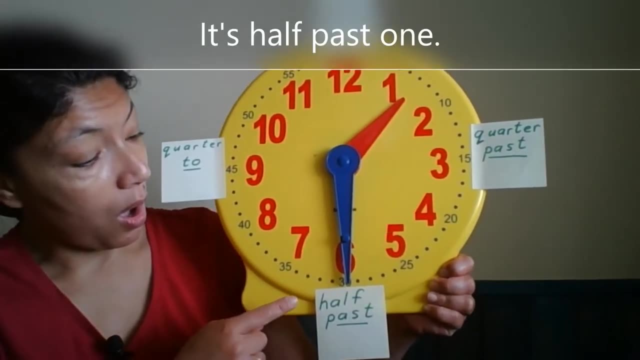 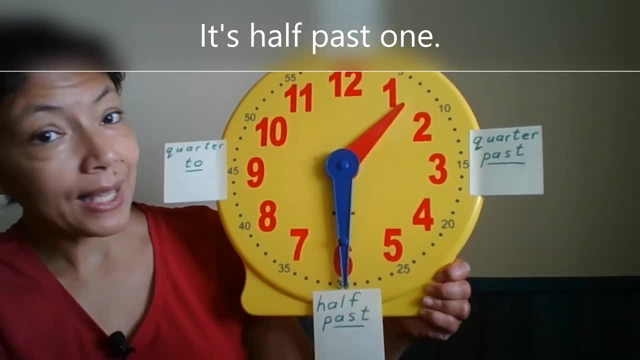 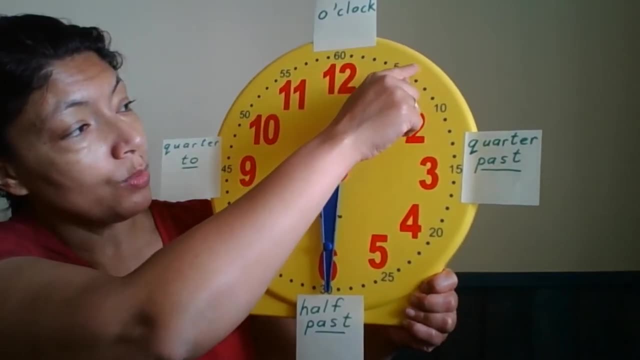 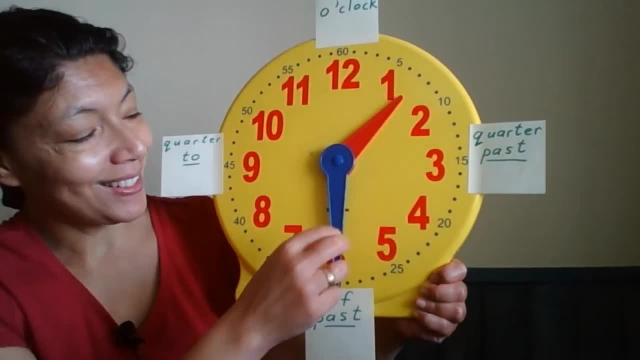 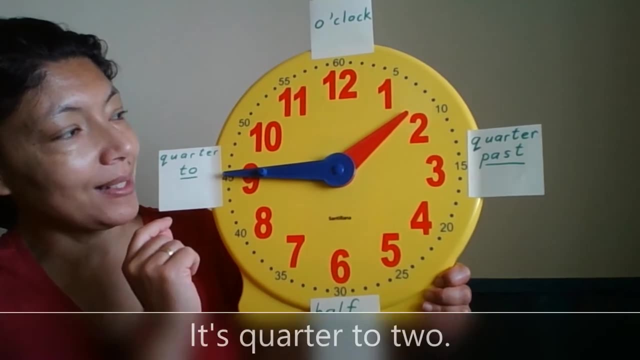 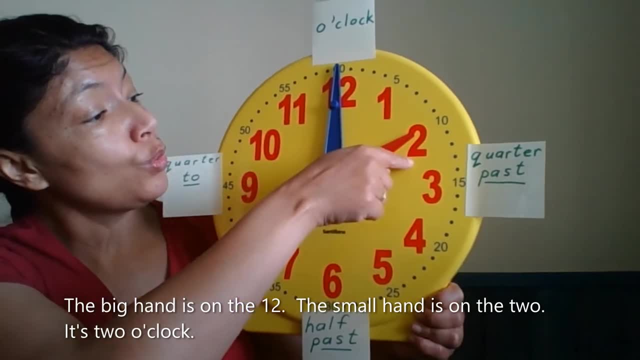 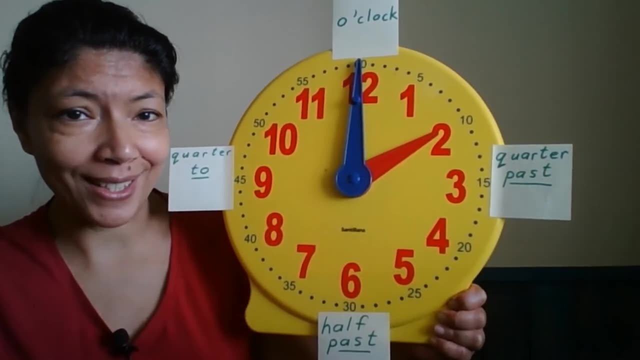 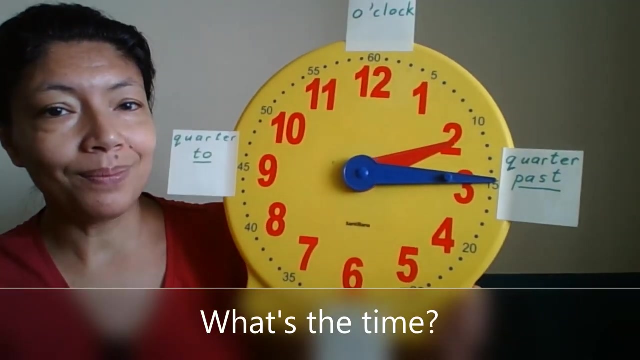 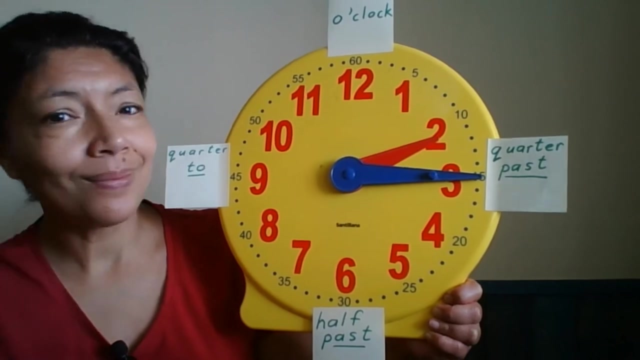 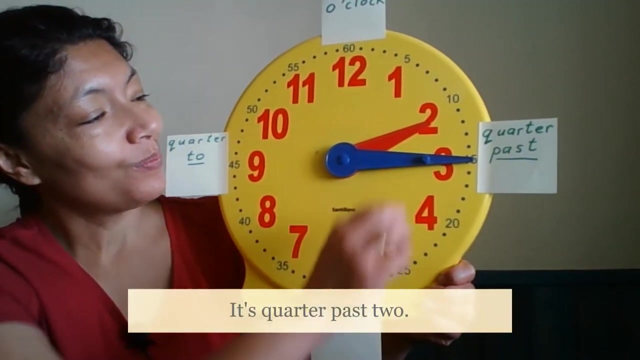 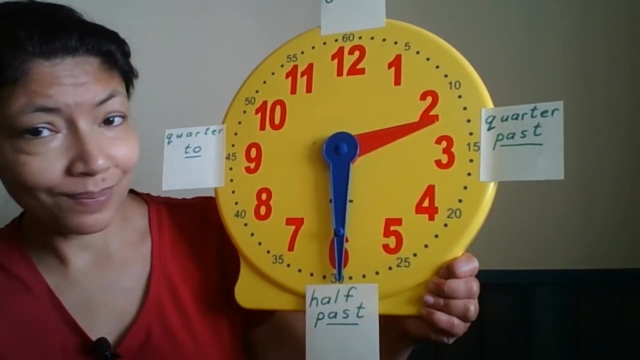 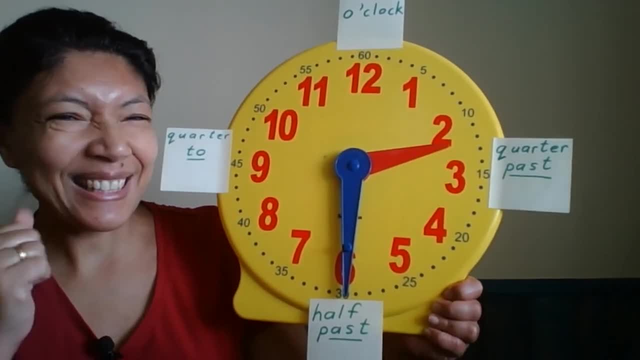 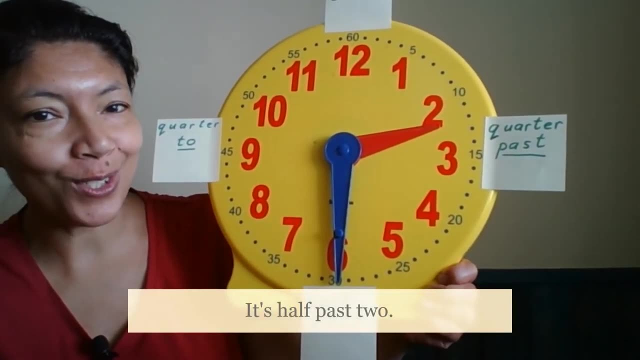 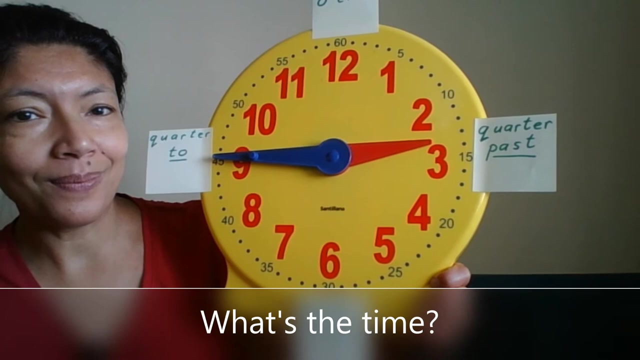 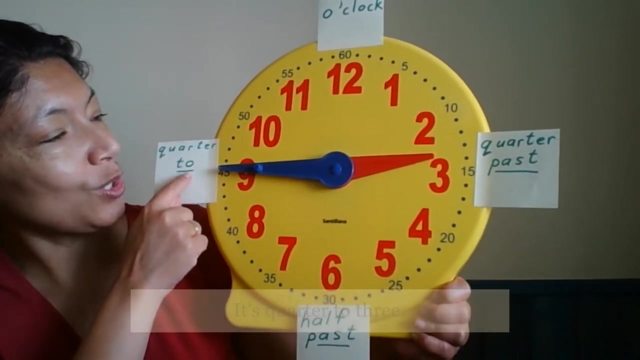 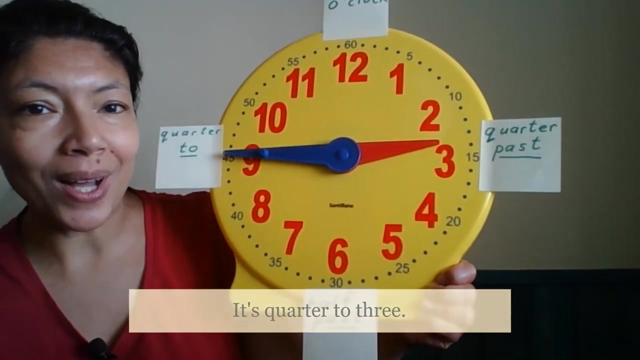 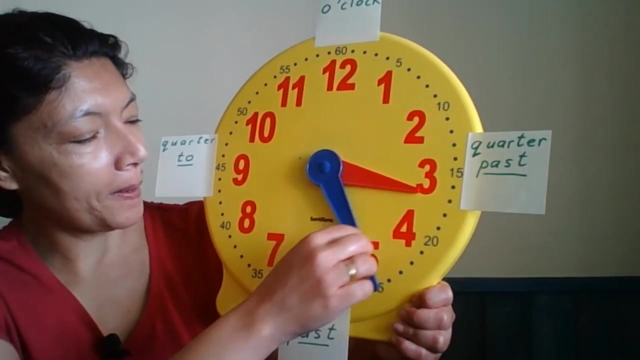 Yes, fantastic, It's half past two. What's the time? Very good, That's right. It's quarter to three. It's quarter to three. You're doing so well. That's great. Let's make this a little bit more difficult. 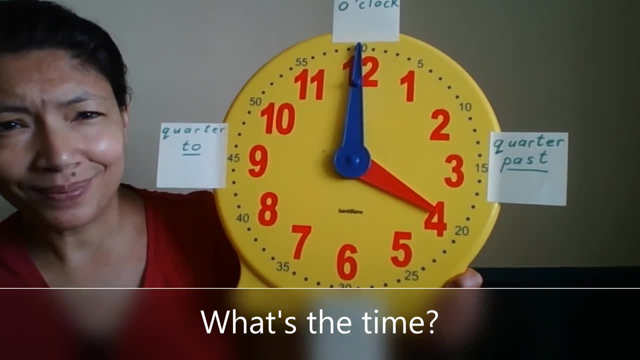 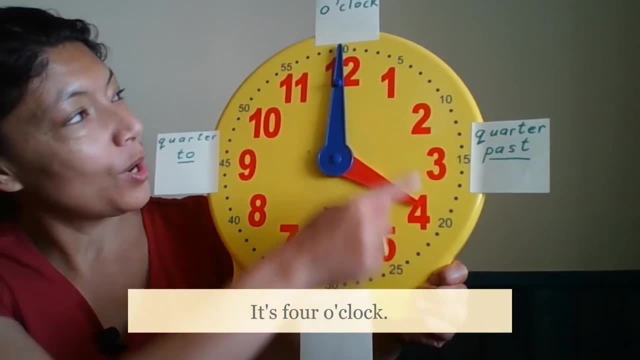 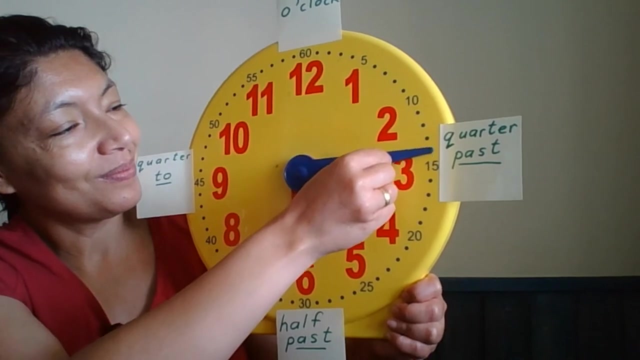 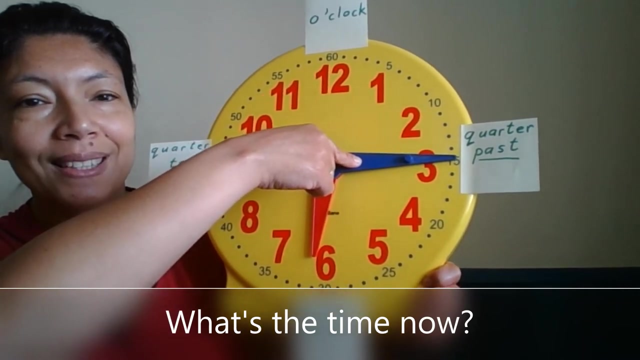 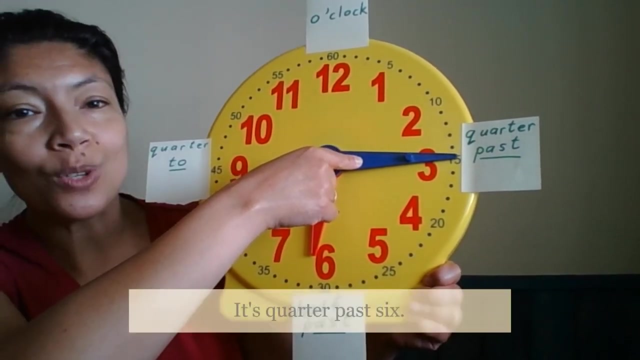 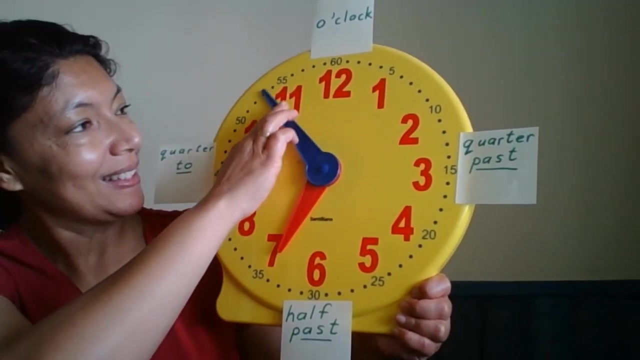 What's the time? Yes, it's four o'clock. It's four o'clock, Yes, correct? What's the time now? What's the time now? Yes, that's right, It's quarter past six. What's the time now? 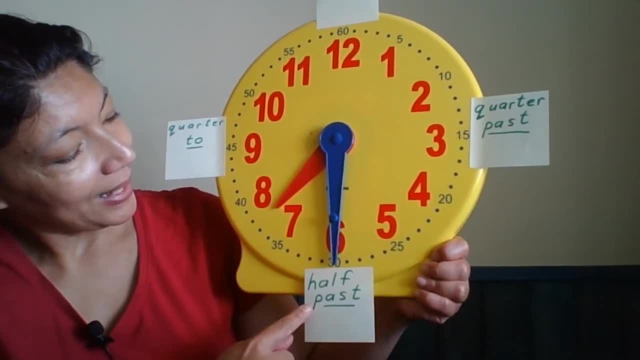 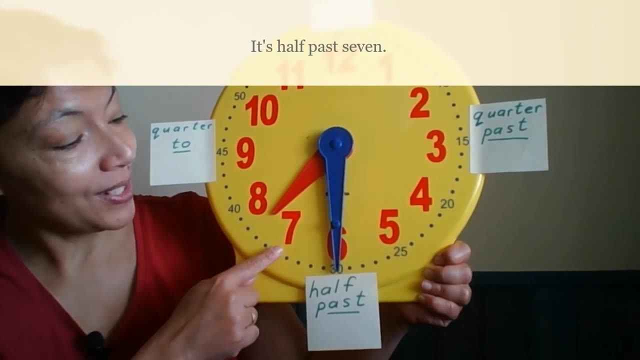 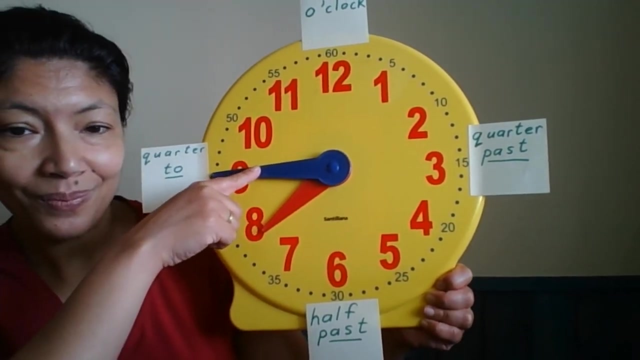 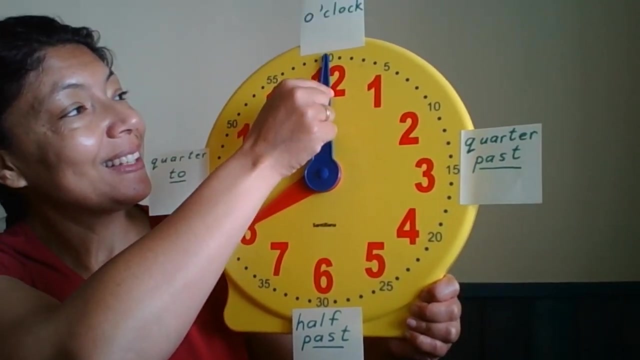 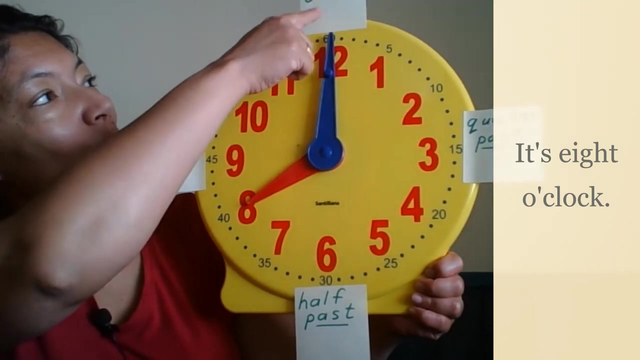 Six o'clock. It's half past seven. It's half past seven. What's the time now? Yes, it's quarter to eight, And now, That's correct, It's eight o'clock. You did very well.